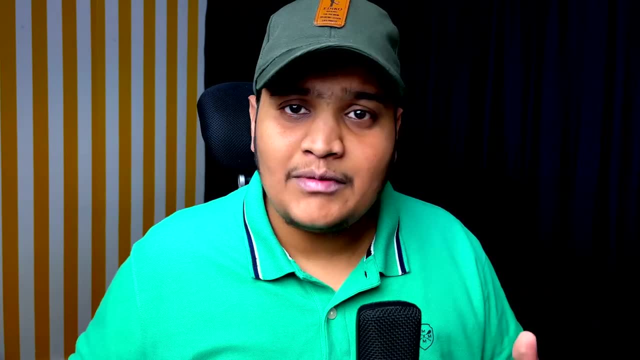 So iterator's job is to allow a client to traverse through the entire data structure based on the data that we have stored in the different data structures- okay, either it may be array, list, tree, whatever it is okay- or, with the iterator, it should allow us to go through the data structures and 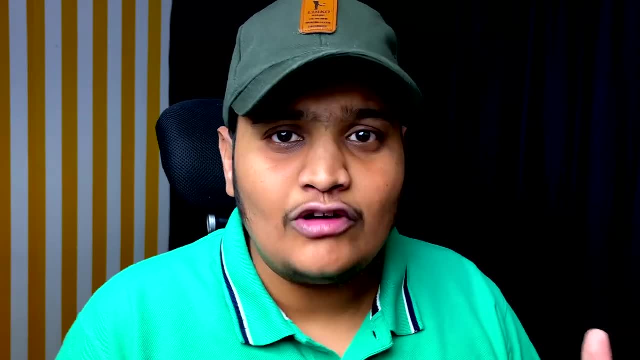 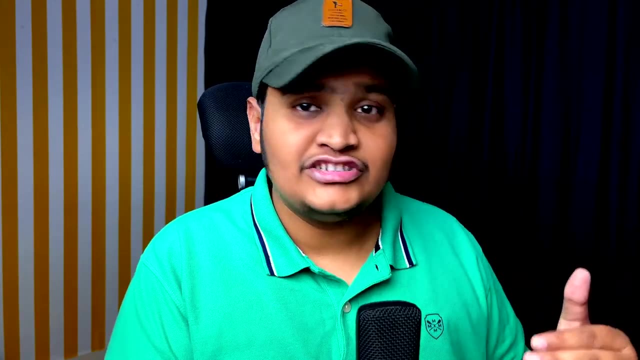 fetch the data. multiple different iterators also should be allowed to traverse through the data. so that's the general idea behind the iterator design pattern. okay, now, as we talked about, like different data structures might have different types of iteration. that needs to be done. there has to be. 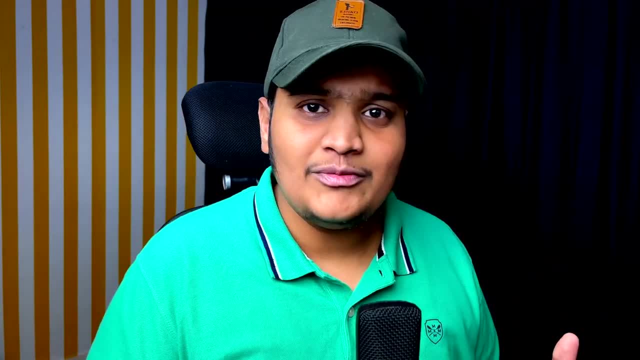 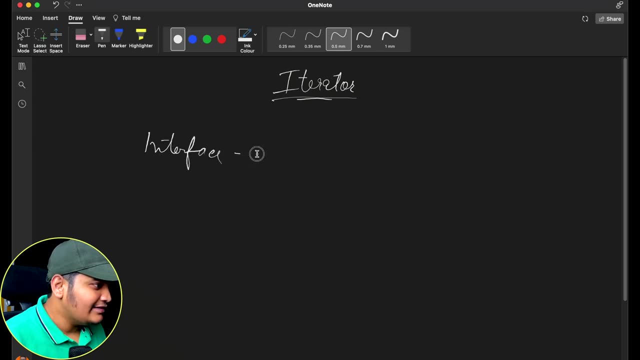 different implementation of the iterator as well. right, so what, generally, we'll be doing is: there has to be an interface of the iterator, okay, generally, it has to be have the interface, and this interface should have the different implementation. right, different implementations. now, this different implementation will be used in the different types of data structures. okay, 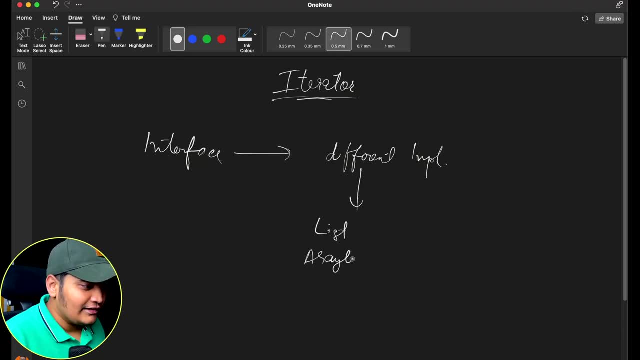 suppose, for list there might be different implementation, for array list there might be different, for trees there might be different, and so on. okay, so for all these different types of data structure, the implementation may vary, but all of them would be be implementing this iterator interface. okay, so this iterator interface will be implemented. 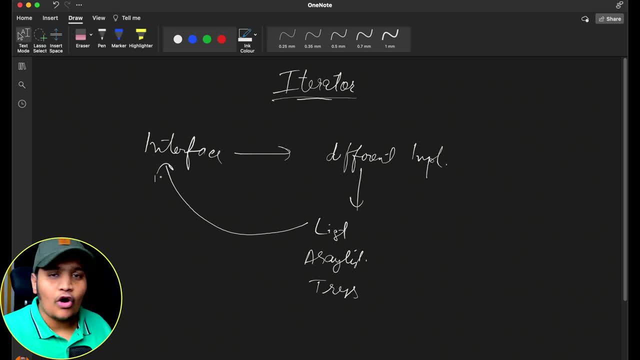 by all of these different interface. so there is no compatibility issue between all these different classes of the collection. now, the best example to see the iterator design pattern is within the collection framework itself, right, so in the collection framework for all these different classes, we can see there is an iterator available and with the help of 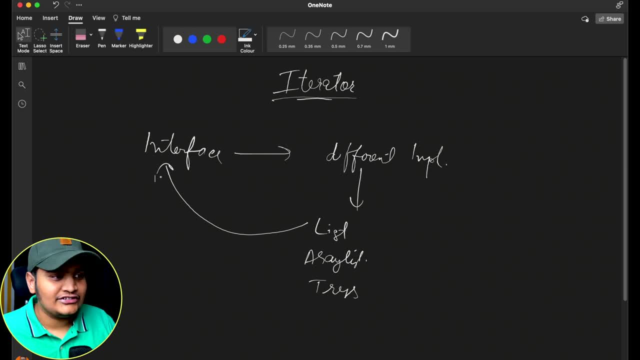 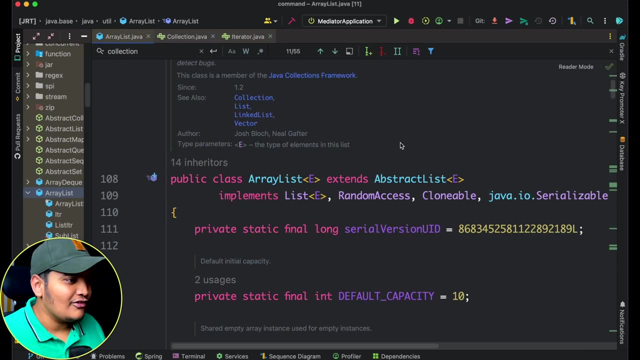 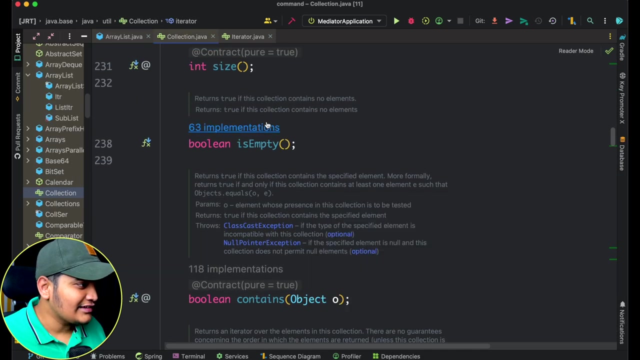 that iterator, we can traverse through the different objects in the collections. so let's see the same example here. let me go through the intellij idea here. okay, and here you can see that we have open the error list. okay, error list is extending abstract error list and it is part of the collection. so if you see this collection interface, right, this collection. 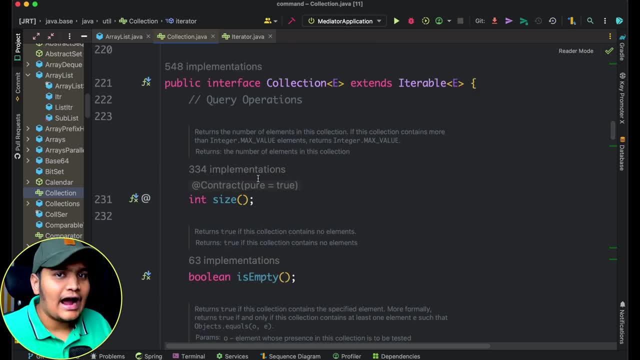 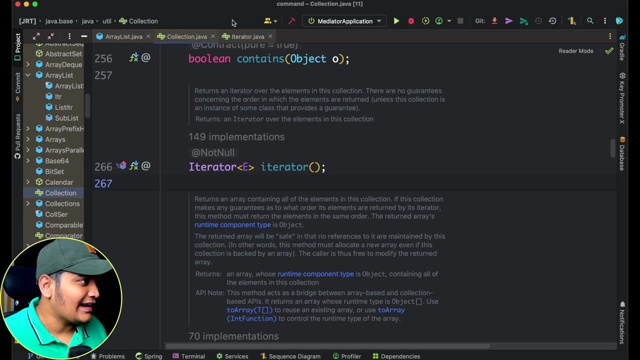 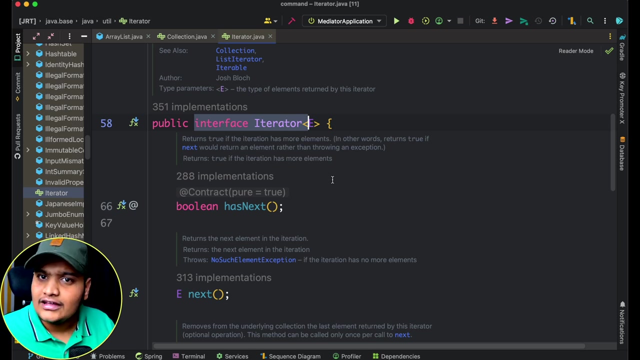 interface is extending iterable, so that means this can be iterated, okay, and that's why it has the object of the iterator, okay. so here you can see that this iterator is the interface, okay, and this iterator will allow us to get the next object of the collection. 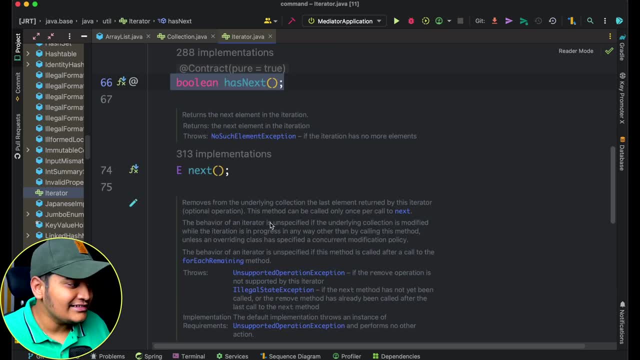 available. So you can see that It has the method that is, hasNext and next, which will check if there is an object available and if so, we should get the particular object as well. So that's the general idea behind the iterator: It should give us the different objects or the next objects available until that particular. 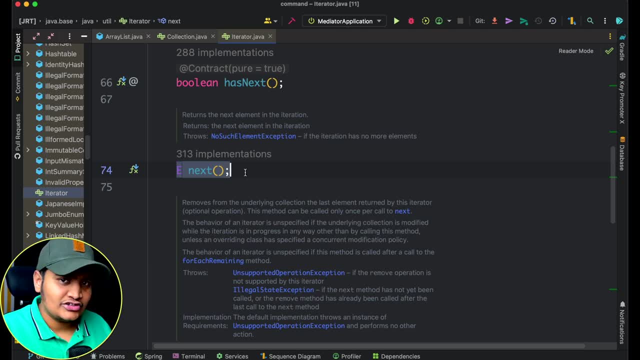 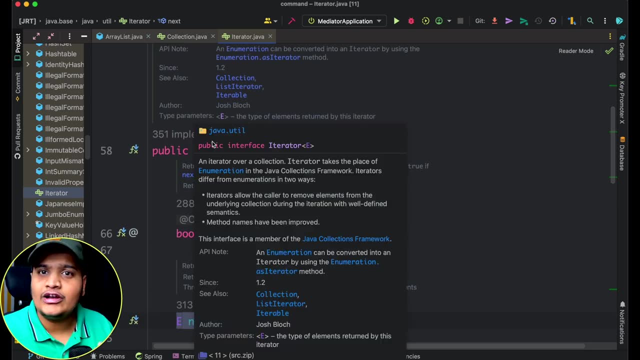 collection is empty. okay, till that, we should get the objects. So that's generally. the iterator should work Now. this is the general interface. you can see, this is the interface. Now this interface should have different implementation based on the different classes of the collection. 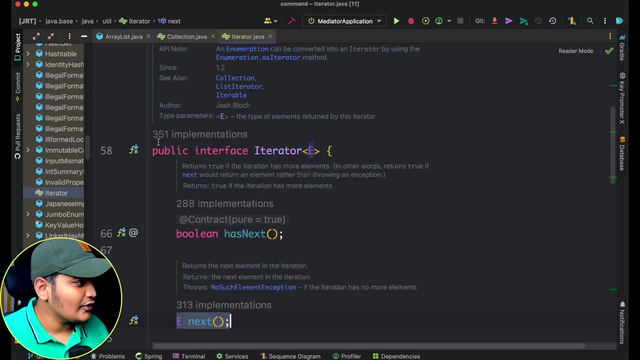 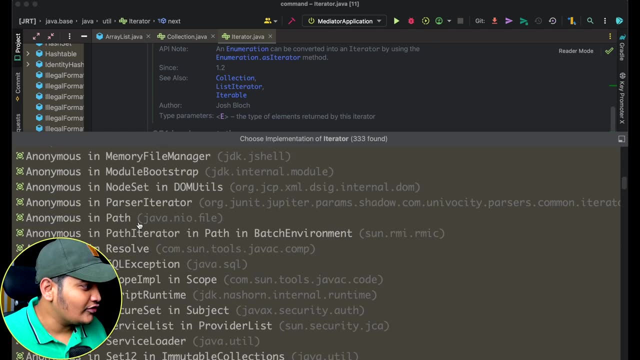 In general for the different concrete classes. okay, So here within the Java you can see that there are 351 implementation for this iterator. So if I just scroll through you can see there are a lot of different implementations for the different collection. here you can see that for list there is one list, adapter list. 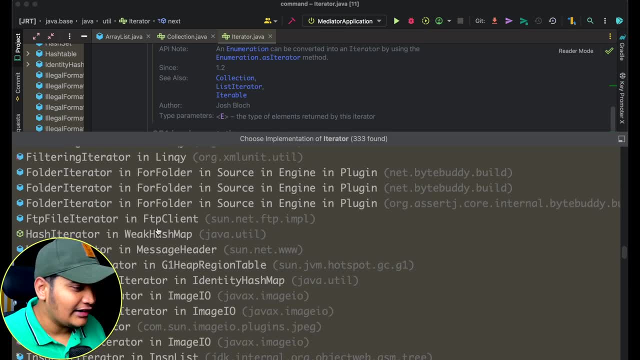 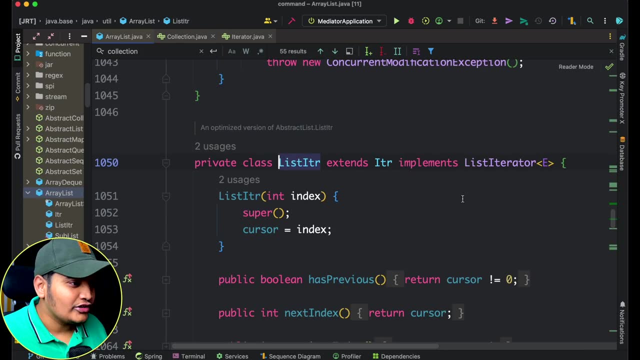 buffer. okay, If I scroll down, you can see there are a lot of different types of implementation available. Let's take the simple one, ArrayList. So there is an implementation for the ArrayList as well for this iterator. okay, So here you can see that it is a simple list iterator which is extending iterator. 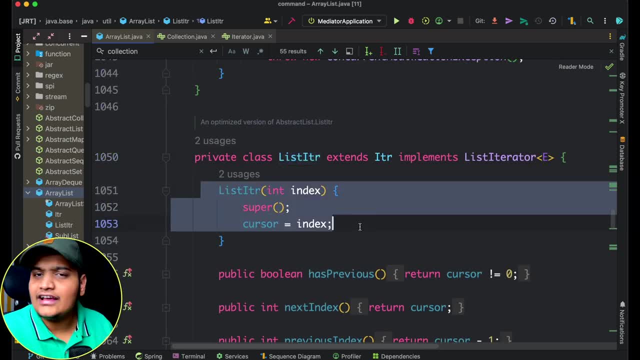 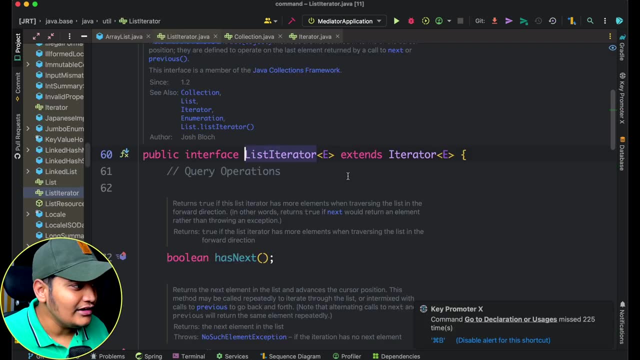 Okay, and it is just, you can see that getting the current index to get the current data, So there might be different implementation. you can see there is a implementation for the list iterator as well, which is extending the iterator, So there are different types of implementation available for the iterator. 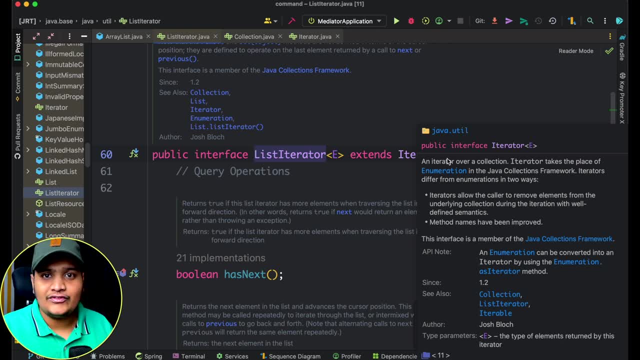 At the end, the main purpose is to have a particular interface and the implementation, concrete classes for that interface which will allow us to traverse to the different objects based on the collection. It might be list of dogs, it might be list of anything, okay, It might be custom data structure as well that you have created. but if you want to traverse, 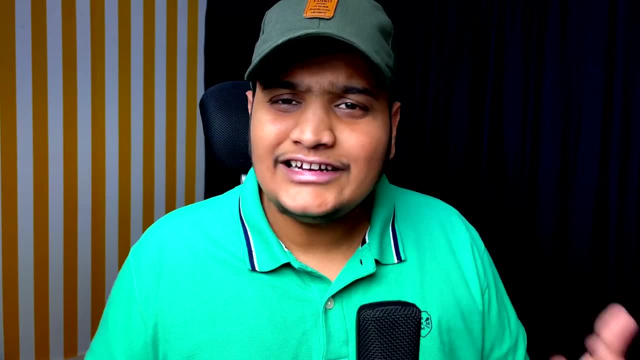 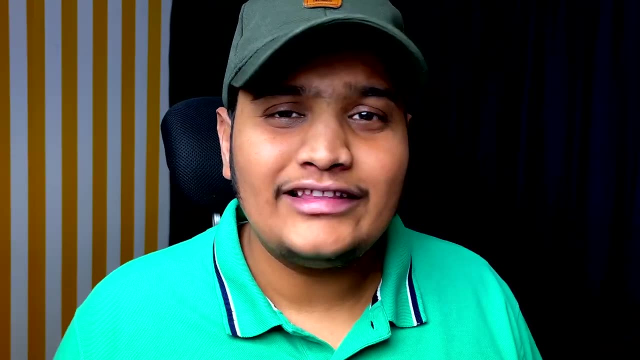 through anything. iterator design pattern is something that you have to implement. So that's the general idea behind the iterator design pattern, and you have seen and used this iterator design pattern a lot in Java as well, So I hope you get the gist around the iterator design pattern and, if you like this video. 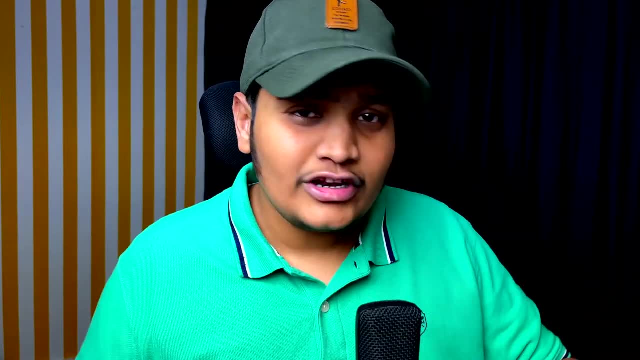 give us a thumbs up and subscribe to my channel for the upcoming videos, and you can also click on the join button to support me as well. I will see you in the next video. till then, happy coding, bye, bye.